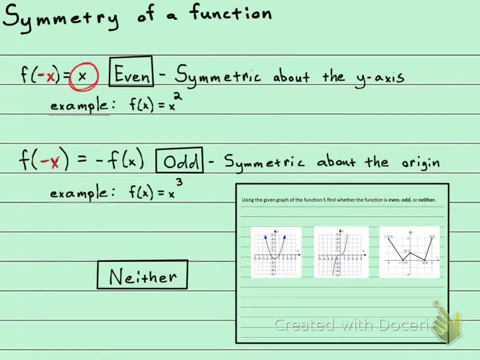 get back is exactly the same as what you started with as your original function, then it's even different. if what you get back is the opposite of your original function, then it's going to be odd. otherwise it's going to be neither. so let's go over and let's look at our example here. 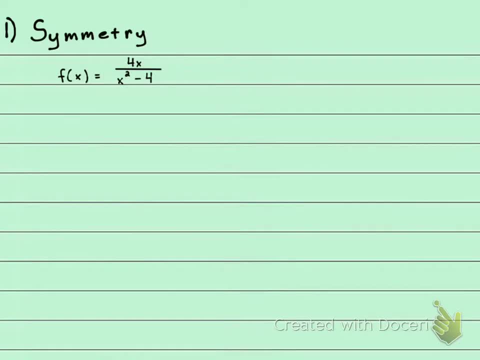 we want to find the symmetry of this function right here, this rational function. so what i need to do is i need to find the f of negative x. i'm going to plug in a negative x everywhere where i saw an x. so this was 4x over x, squared minus 4.. i'm going to plug in a negative x. 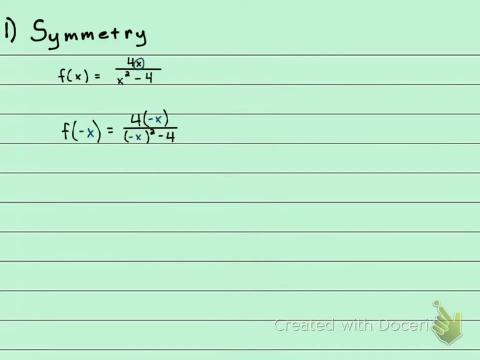 on top and a negative x on the bottom. okay, everywhere where i saw an x, i'm now plugging in the negative x. okay, and let's see what happens in numerator. i'm going to get negative 4x in the denominator. this is negative x squared. so that's a negative times, a negative, negative x. 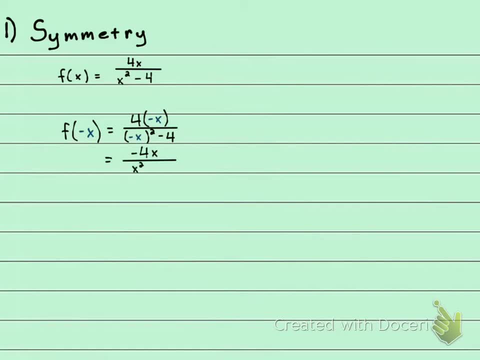 times negative x is positive x squared minus four. all right, so let's look at this. is this exactly the same as this one? and the answer is no. it's not exactly the same. now, is this the exact same one? is our first 2x over x squared minus 4? so the answer is this: the exact opposite of this. 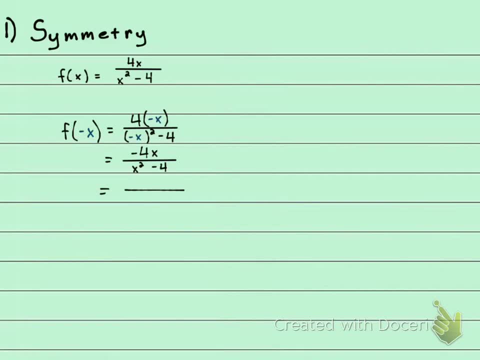 and the answer to that is yes. if i rewrite this and i take this negative in the numerator and i pull it out in front, it's going to be the opposite of 4x over x squared minus four. so i'm going to have the opposite of what i think of. x is negative, x squared minus 4 into negative x, and so i'm going to take negative x here and leave everything part of x in Portable. 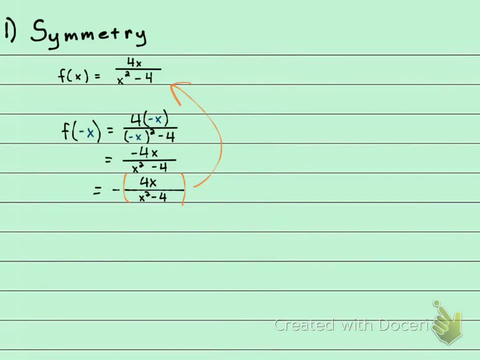 of what I started with. So this is going to be odd, Okay, which means that it is symmetric about the origin. Alright, that's the first part. Let's go look at the second step.